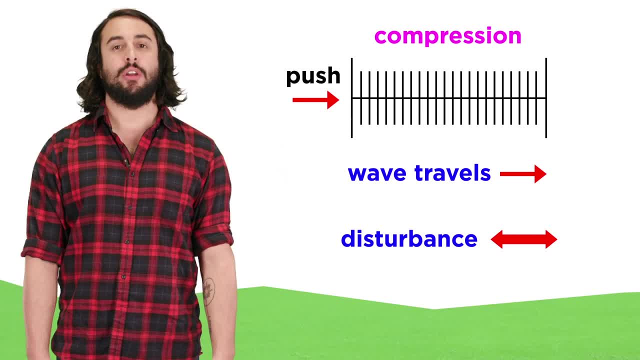 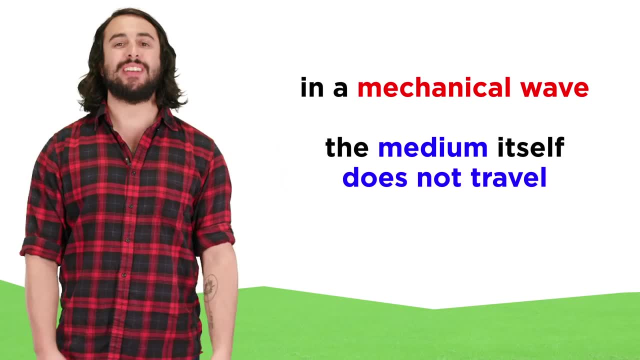 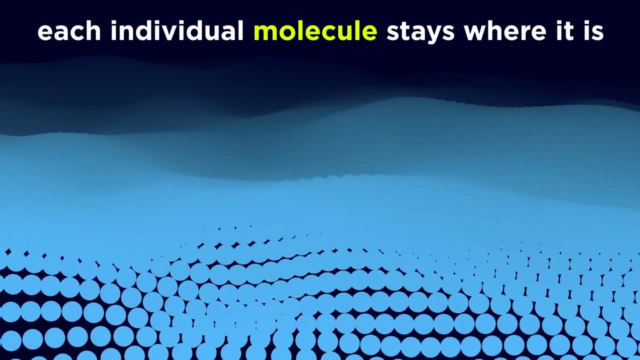 the direction the wave is traveling, either by compression or rarefaction. With mechanical waves the medium does not travel with the wave, just the energy is carried by the wave. So in the ocean the wave will travel a great distance. but any individual water molecule 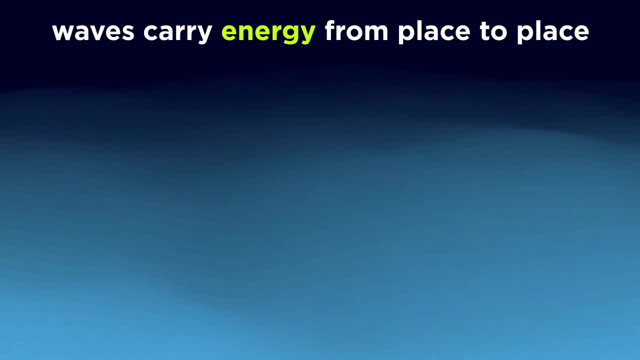 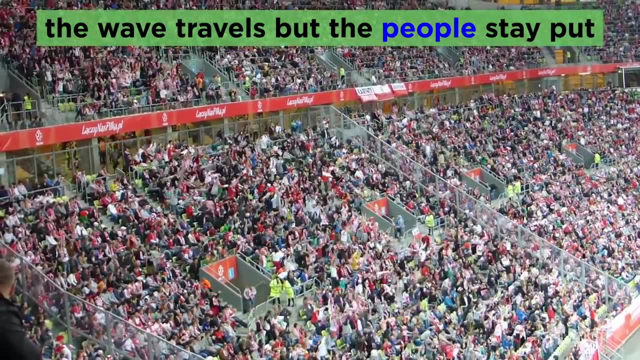 won't go too far. it is only energy that travels along with the wave. The same can be said for people doing the wave at a stadium. The wave travels, but all of the people stay in their own seats. However, not all waves are mechanical waves. 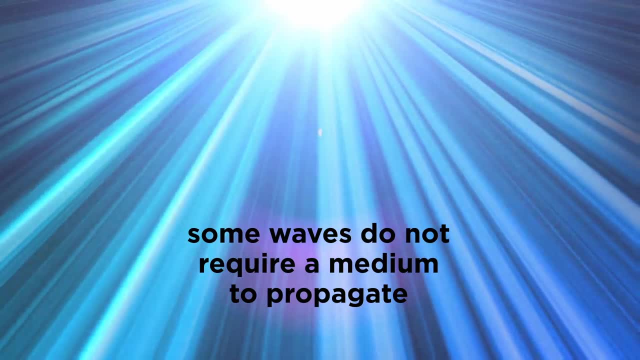 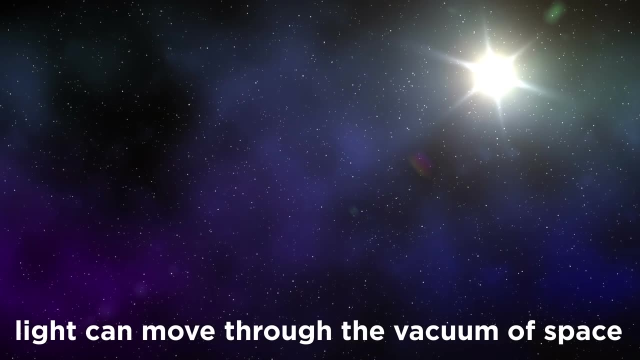 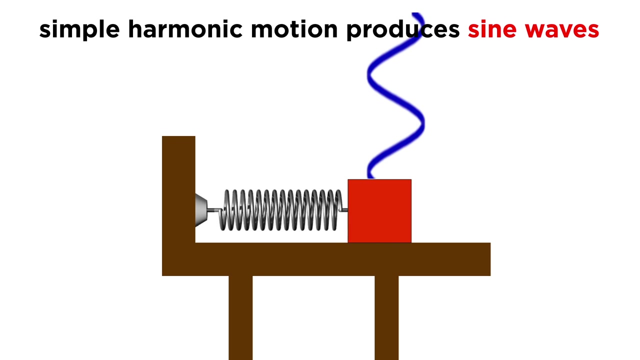 Some do not require a medium to travel through. like any kind of electromagnetic wave which we know of as light, These waves can travel through the vacuum of space, which is why we are able to see celestial objects in the night sky. A wave whose source is a vibration with simple harmonic motion will be a sine wave, because 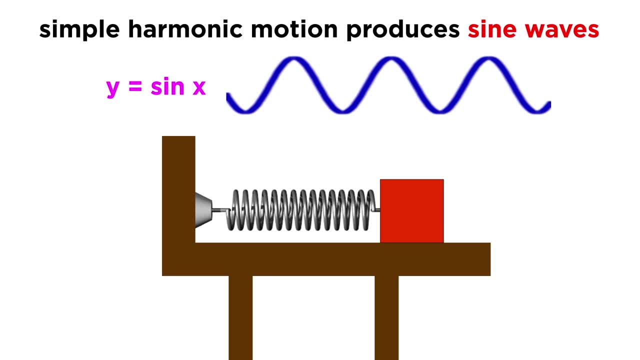 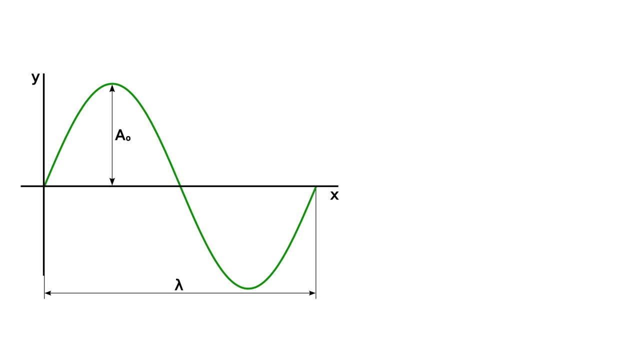 the periodic motion of the wave produces a graph of the trigonometric function. Y equals sine X. We need to label a few details with sine waves. First there is the amplitude of the wave. For a transverse wave like this, the amplitude is the displacement of the wave in the direction. 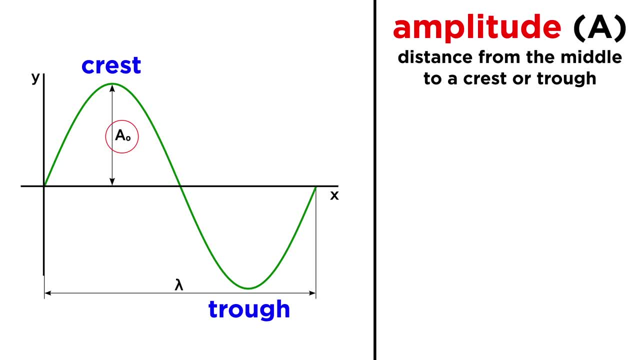 perpendicular to the direction of its motion or the distance from the middle to a crest or trough. The greater the amplitude, the more energy the wave carries with it, which is why you shouldn't try to surf 30 foot waves unless you are an expert. 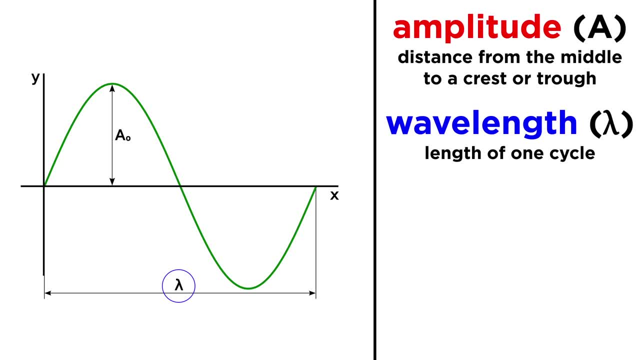 In addition, each wave will carry a sine wave. The amplitude of the wave is the displacement of the wave in the direction perpendicular to the direction of its motion, or the distance from the middle to a crest or trough. This is called a wavelength, represented by the Greek letter lambda. 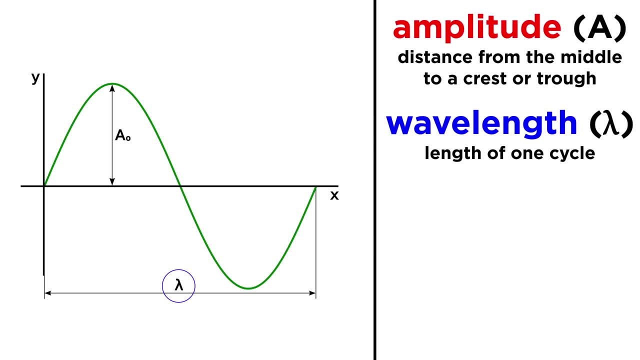 This is the length of one cycle of the wave, which is easily measured from one crest to the next. The time required to complete one cycle is called the period. There will also be a frequency, which is the number of wavelengths that pass by a particular. 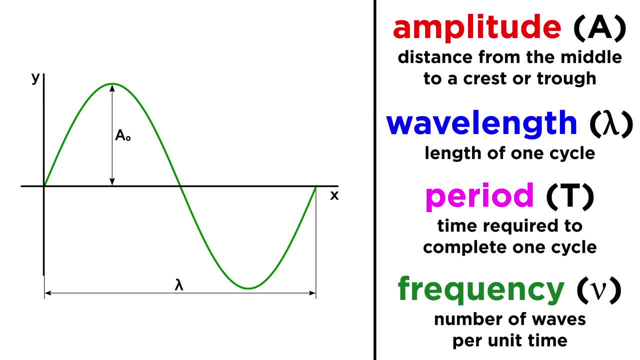 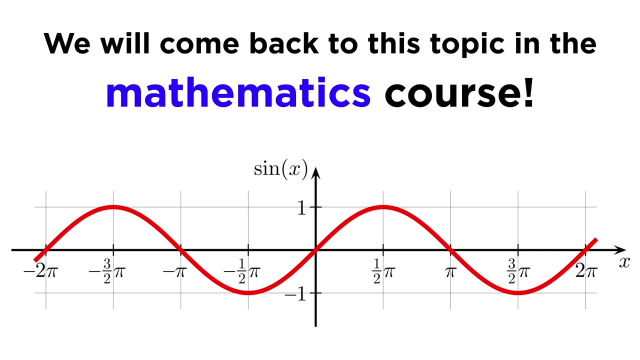 spot per unit time, represented by the Greek letter nu. Frequency will typically be measured in hertz. We will learn all kinds of math associated with graphing these sine curves in the upcoming mathematics course. For now, we can just stick to a qualitative discussion. 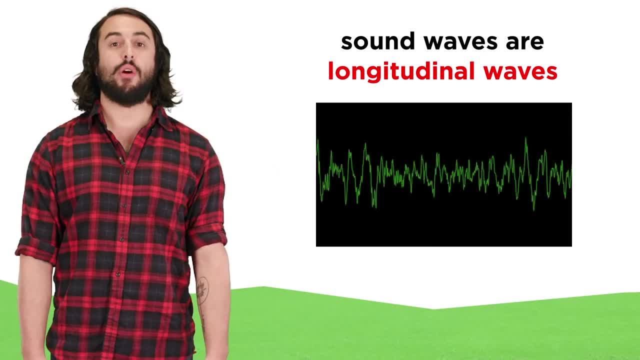 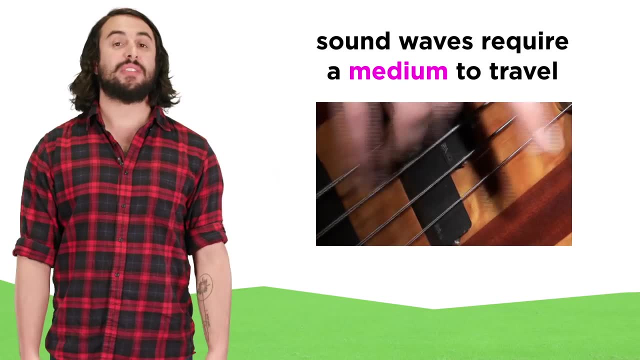 Sound is also brought to our ears through waves, though these are longitudinal waves. A sound initiates with a vibration, like a plucked string. This vibration requires a medium in order to generate a sound. It requires a medium in which to travel, like a solid liquid or gas. 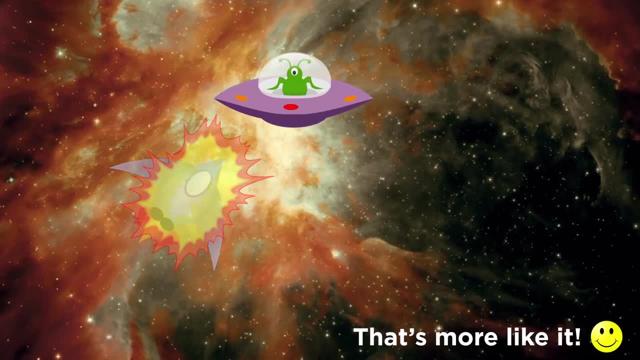 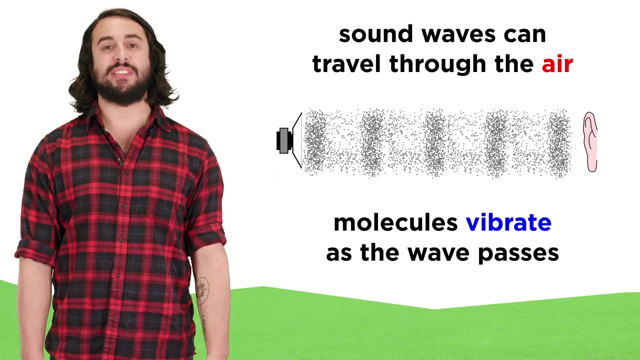 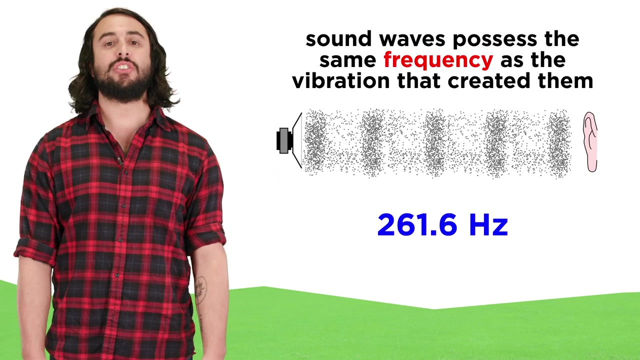 Sound can't travel in a vacuum, which is why there is no sound in space, despite what you hear in movies. Typically, sound travels through the air, causing vibrations in atmospheric molecules as it passes, just like a wave in the ocean does to water molecules. 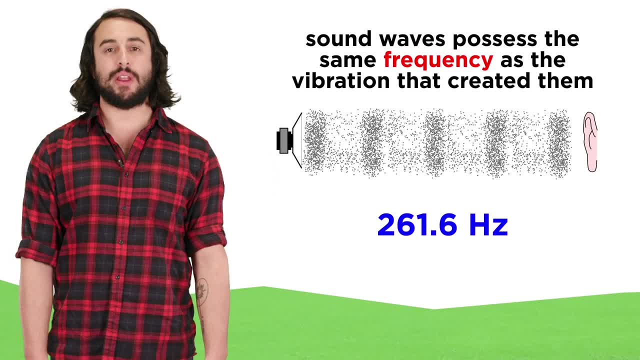 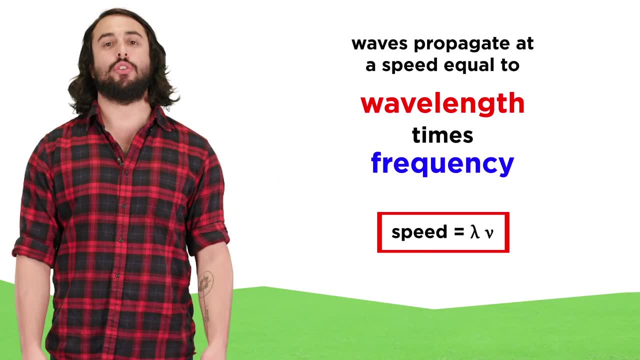 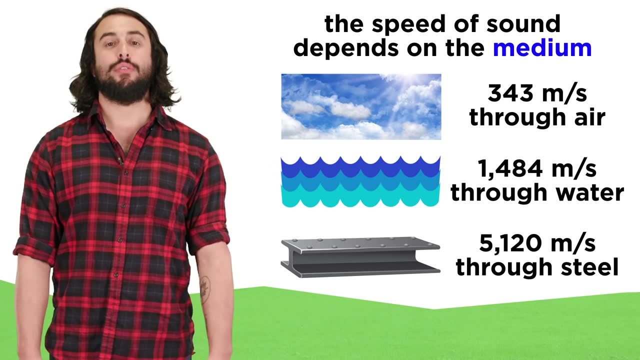 Each sound wave will carry a frequency that is equal to the frequency of the vibration that initiated it. The speed at which the wave will travel is equal to the wavelength times. the frequency and mechanical waves will travel at a constant speed for any given medium, though that speed. 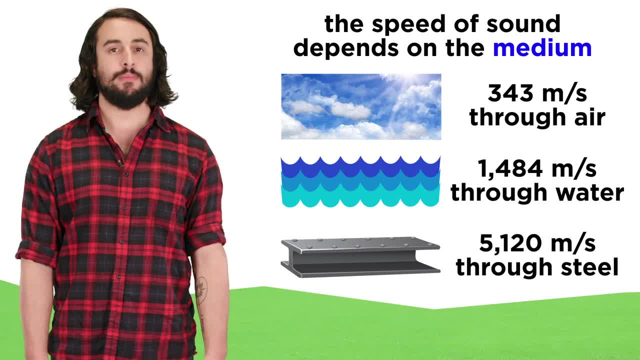 is different depending on the particular medium. Interestingly, sound travels four times faster in water than air and seventeen times faster through steel than air. But when we refer to the speed of sound, we typically mean as it moves through the atmosphere. Sound travels four times faster in water than air and seventeen times faster through steel. 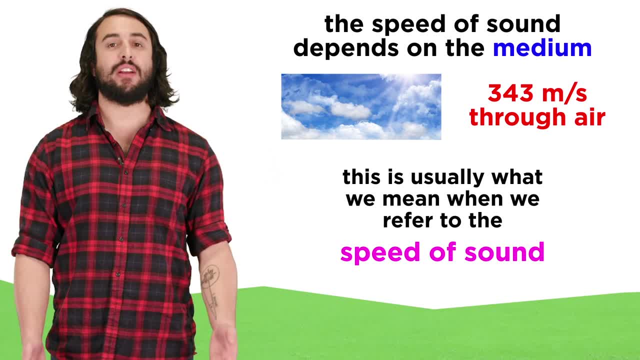 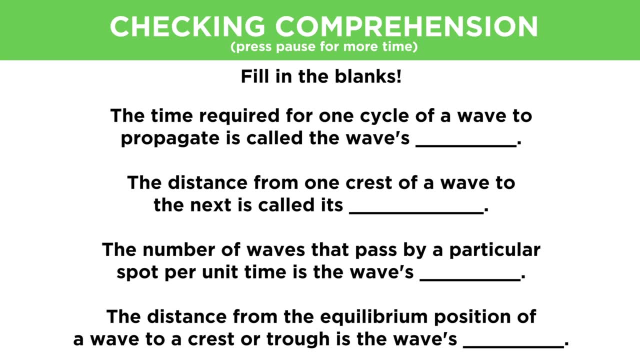 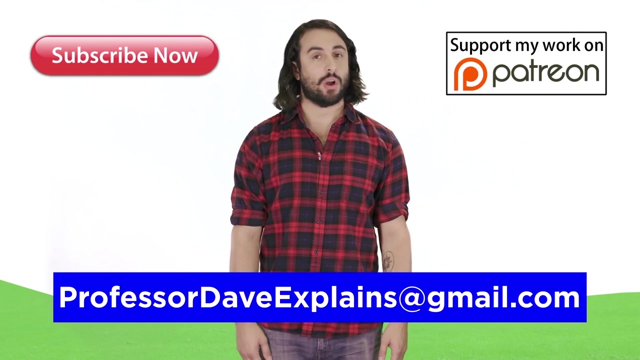 than air. The same happens to the autumn atmosphere, which will be constant, since a greater frequency will be accompanied by a smaller wavelength. Let's check comprehension. Thanks for watching, guys. subscribe to my channel for more tutorials. support me on patreon so I can keep making content and, as always, feel free to email me. 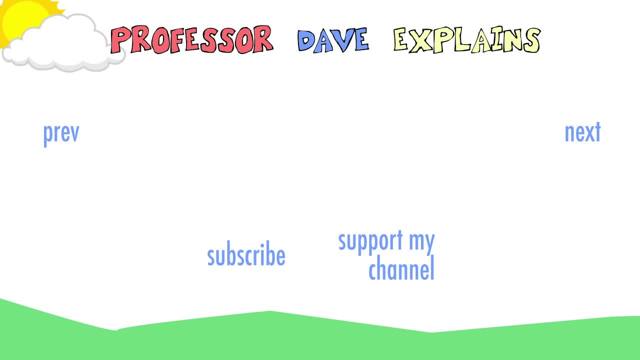 and I'll see you in the next one.